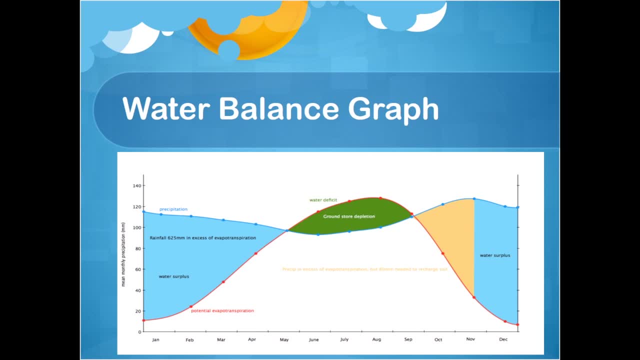 us two things: that more moisture is entering the atmosphere than leaving, which leaves us with a deficit that is compensated for by groundwater storage. When precipitation is once again higher than evapotranspiration, we see a period of recharge where the groundwater is replaced before we are back to surplus again. 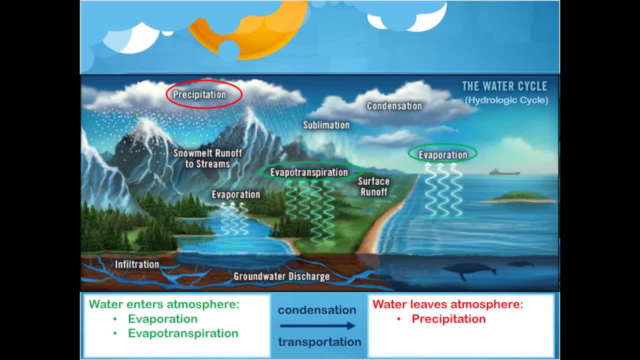 Let's look at the water cycle and try to guess what the impact of evapotranspiration is on the water budget. Let's look at the water cycle and try to guess what the impact of evapotranspiration is on the water budget. Inflows and outflows would be in the water budget as we go through the steps of the water. 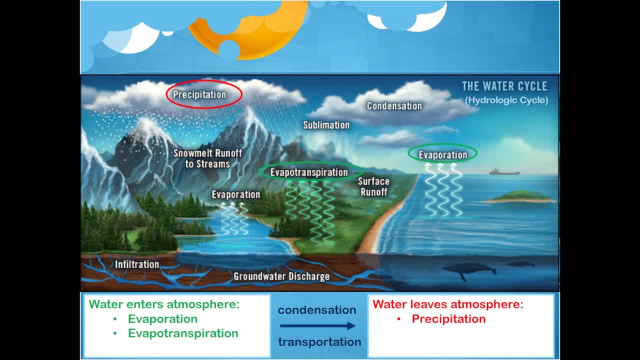 cycle. Water enters the atmosphere through evaporation and evapotranspiration. Once the water is in the atmosphere, it undergoes condensation and transportation before becoming precipitation and leaving the atmosphere. Evaporation and evapotranspiration are always outflows and precipitation is always an inflow Groundwater. 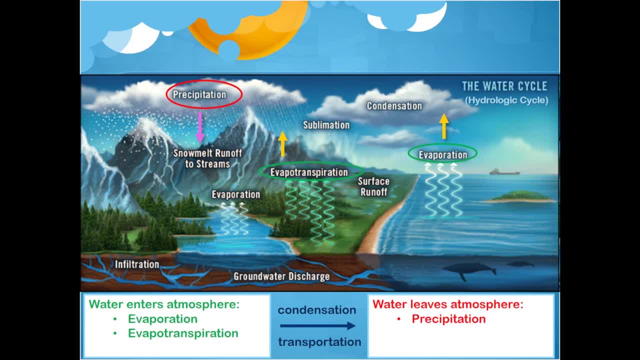 discharge and streamflow are always outflows. Groundwater discharge and streamflow are always outflows, and precipitation is always an inflow. Groundwater discharge and streamflow are always outflows, depending on whether more water is entering or leaving the system. 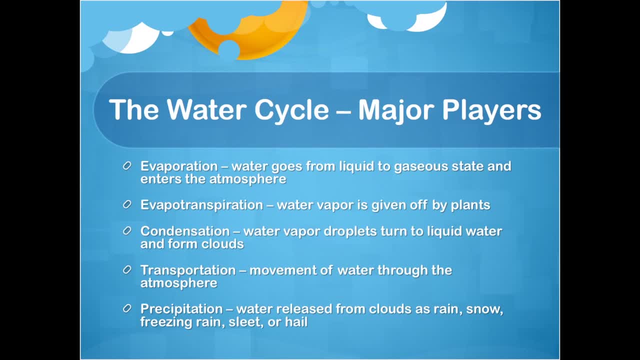 Before we continue with the water budget, let's define the major players in the water cycle. Evaporation occurs when water goes from liquid to gassy state and enters the atmosphere. Evapotranspiration is similar, but the water vapor is given off by plants. 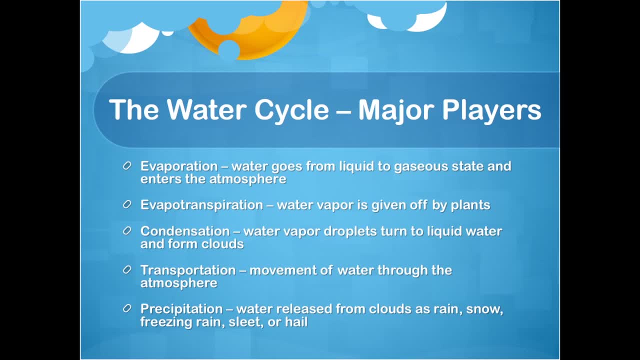 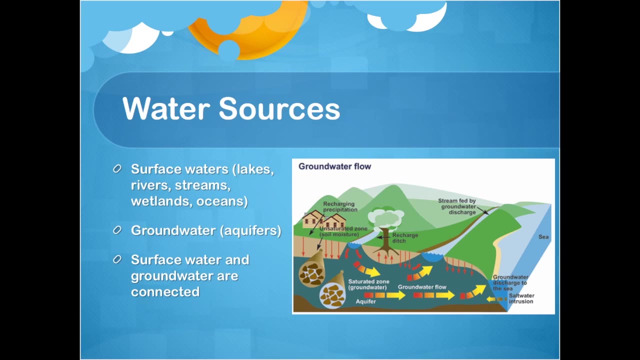 Condensation occurs after water vapor enters the atmosphere. At this stage, the water vapor droplets turn to liquid water and form clouds. Transportation describes the movement of water through the atmosphere, and precipitation occurs when water is released from the clouds. Water that enters the system as precipitation either ends up in surface waters like lakes. 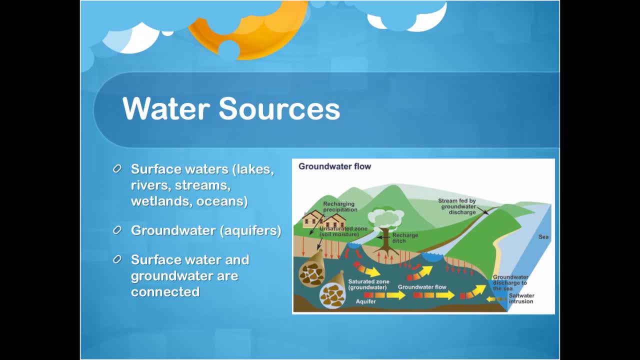 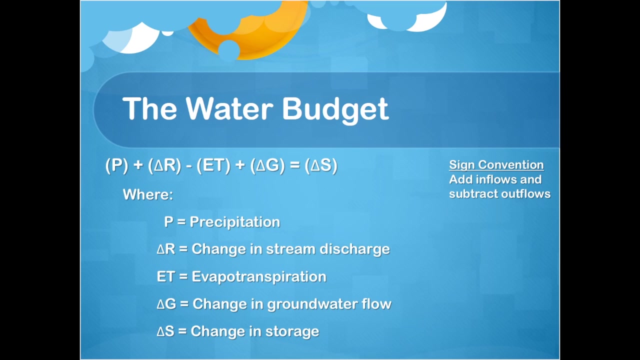 rivers, streams, wetlands or the ocean or groundwater. We'll see shortly that surface water and groundwater are treated as two separate entities in the water budget, but it's important to remember that they are connected. Now that we know a little bit about the water cycle, we can break down the inflows and outflows. 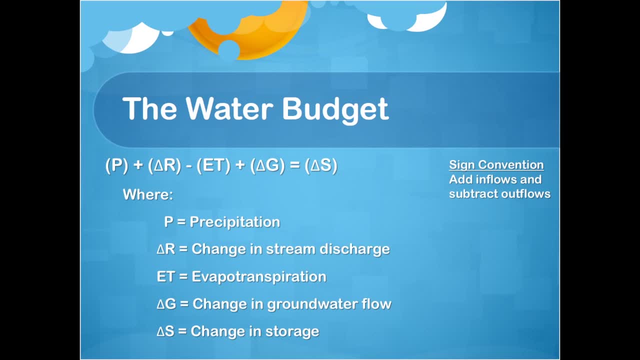 into the water budget equation shown here. The water budget equation tells us that the change in storage is determined from precipitation, change in stream discharge, evapotranspiration and change in groundwater flow. Whether we add or subtract the terms depends on whether they 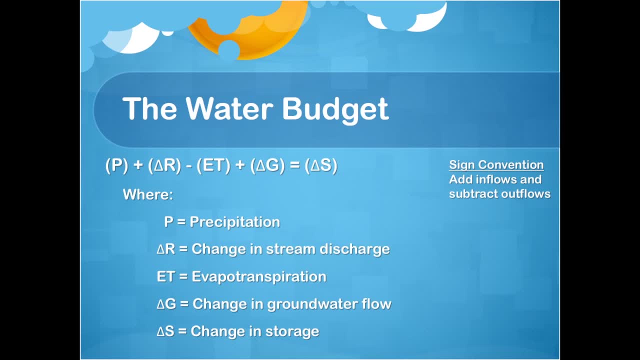 are classified as inflows or outflows. Evapotranspiration is always subtracted because we know it's an outflow, but change in stream discharge and change in groundwater flow can be either added or subtracted depending on the situation. We can simplify the water budget calculation for a watershed that doesn't have 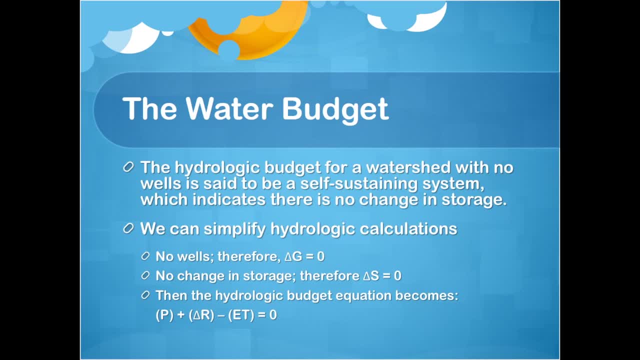 wells and is self-sustaining. No wells means we can assume there is no change in groundwater flow and self-sustaining tells us that there is no change in storage. Then we can rewrite the water budget equation to state that precipitation plus the change in stream, discharge minus the evapotranspiration equals zero. 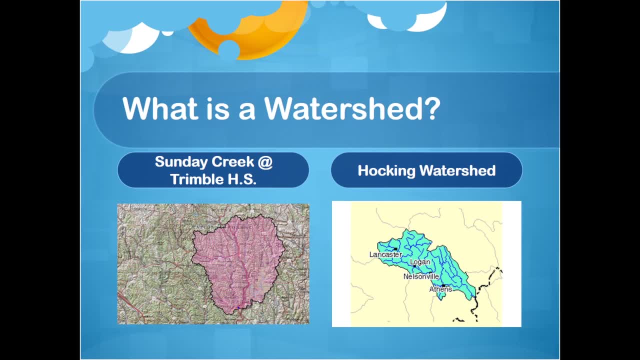 Before we go much further with our water budget discussion, let's take a moment to define watersheds, since this is the closed system that's being considered when we calculate a water budget. Here we have two examples of watersheds: The Sunday Creek Watershed at Trimble High School. 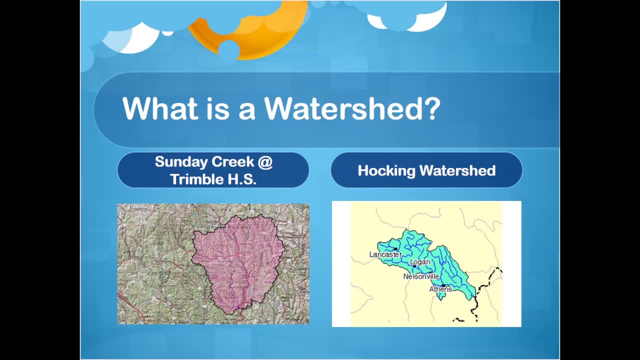 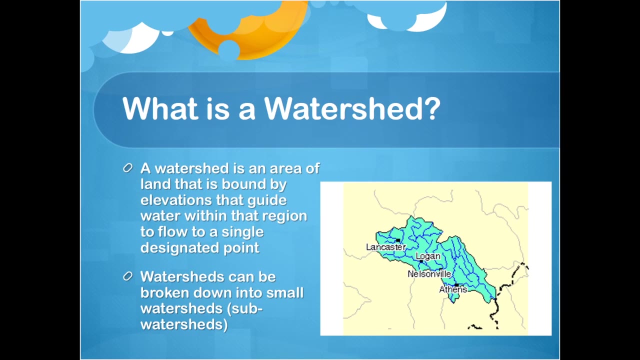 in Gloucester, Ohio And the Hawking Watershed in Southeast Ohio. Looking at these two pictures, how would you define a watershed? Take a few minutes to discuss. A watershed is defined as an area of land that is bound by elevations that guide water within. 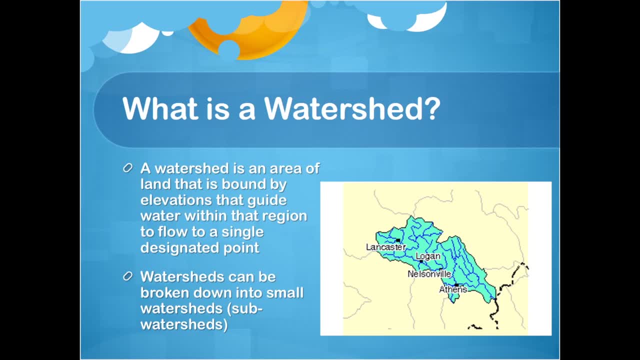 that region to flow to a single designated point. What does all that really mean? This definition is telling us that. This definition is telling us that all drops of water that fall anywhere within this region will eventually end up at the same point, at the end of the watershed, If the water droplet falls outside the watershed boundaries. 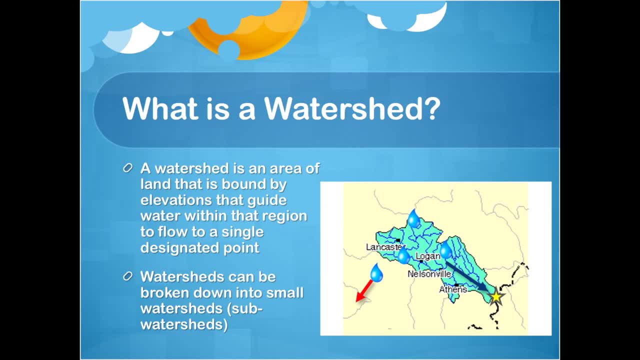 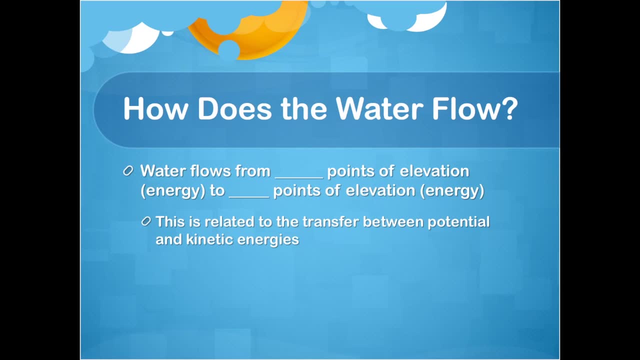 it is part of a different watershed and flows to a different point. Now the question becomes: how do we know which way the water will flow? If we take a walk through the woods, we won't come across a watershed boundary conveniently placed to tell us which way the water will flow. So how do we even begin to? 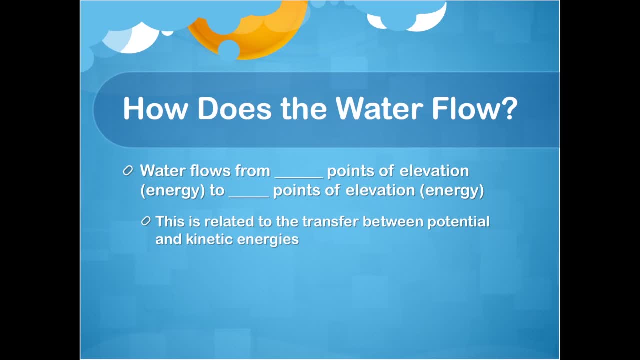 delineate this watershed. boundary Water flows from blank points of elevations or energy. Elevation and energy are used interchangeable in this statement because the answer deals with the concept of potential and kinetic energy transfer. Try to fill in the blanks. Come on, follow me. 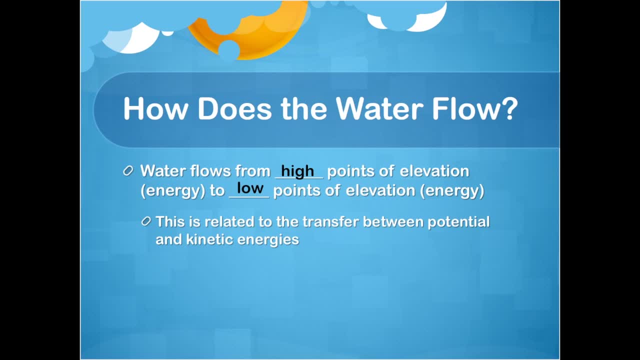 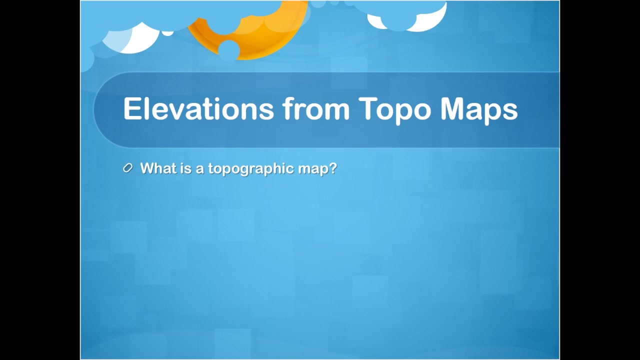 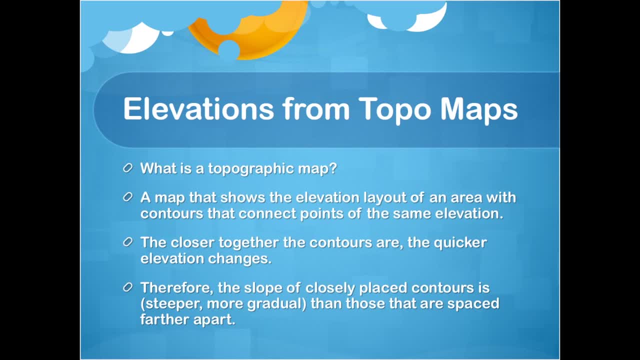 Topographic maps, or topo maps for short, show the elevation layout of an area using contour lines that connect points of the same elevation. Contours that are close together indicate quick changes in elevation. Do you think the slope of closely placed contours is steeper? 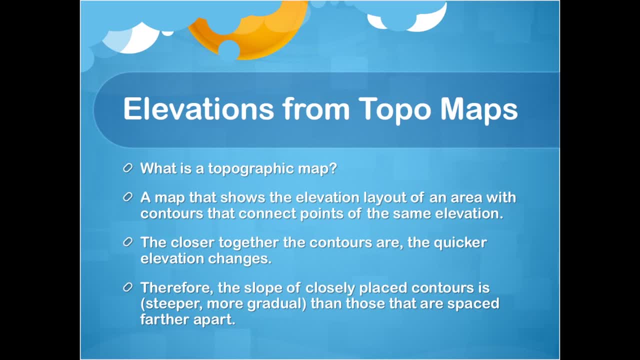 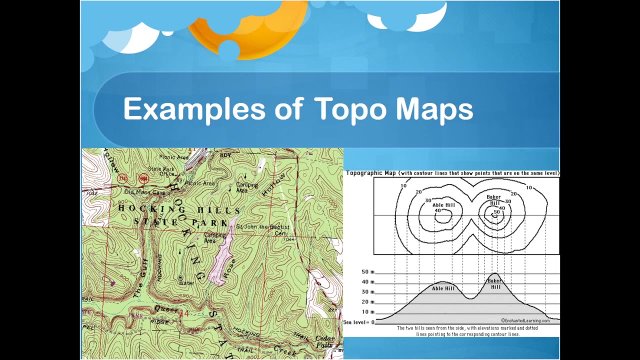 or more gradual than contours that are spaced farther apart. Contours that are close together indicate a steep slope. Let's look at some examples of topo maps. On the left side we have a section of USGS map for the Hocking Hills State Park region in Ohio. 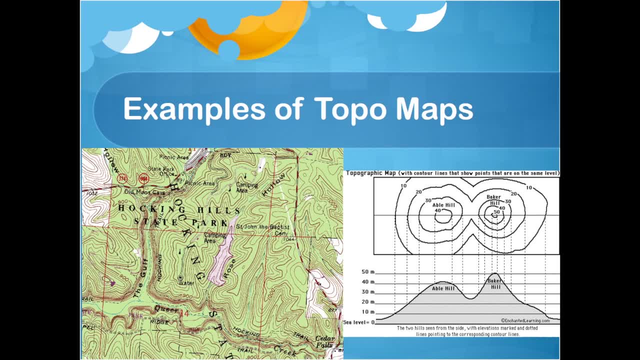 The contours are labeled every 100 feet and each contour represents a 20 foot change in elevation. We can tell that this region on the right side is much steeper than the region on the left side of the map. If we wanted a profile view of a region, we could plot the elevations based. 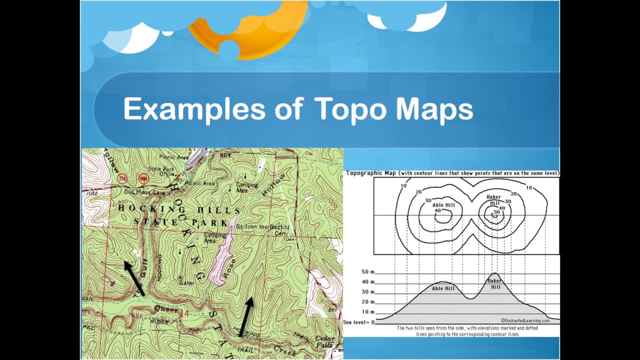 on the horizontal spacing between the contours, as shown in the picture on the right. In doing so, we get an idea of what the area looks like. The contours on a topo map give us an idea of the slope, elevation, slope and water flow. Contours point upstream in valleys and point down ridges. 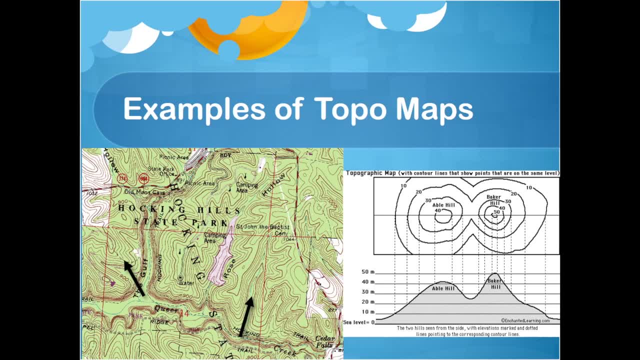 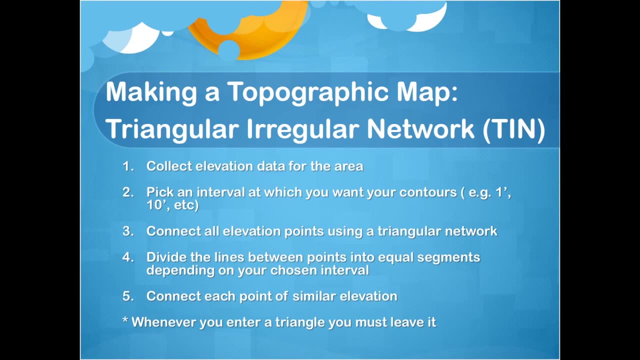 How do you think topo maps are made? Take a few minutes to discuss your ideas. Topo maps can be hand drafted using the triangular irregular network or TIN method. The TIN method involves five steps. First, elevation data needs to be collected through a land survey of the area. 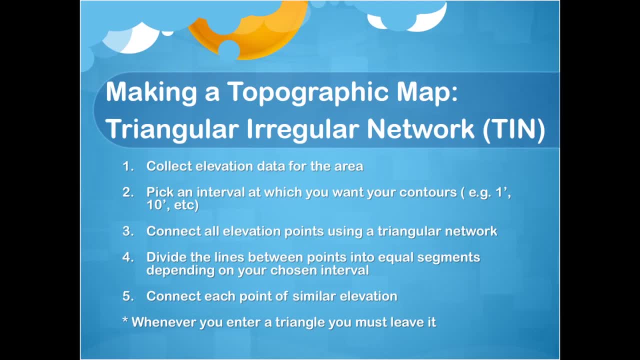 With elevation data points known, the next step is to pick an interval for the contours. Typical intervals can be 1 foot, 10 foot or 100 feet. like we saw in the USGS map, The contour interval size will depend on the scale of the project. 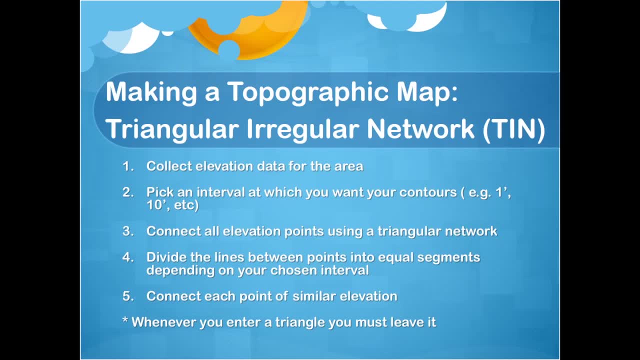 Smaller regions might be mapped in 1 foot or 10 foot intervals, but large areas are mapped in 100 foot intervals. The third step involves connecting all the elevation points using a triangular network. Once all the points are connected, the fourth step divides the lines into equal segments based on the chosen contour interval. 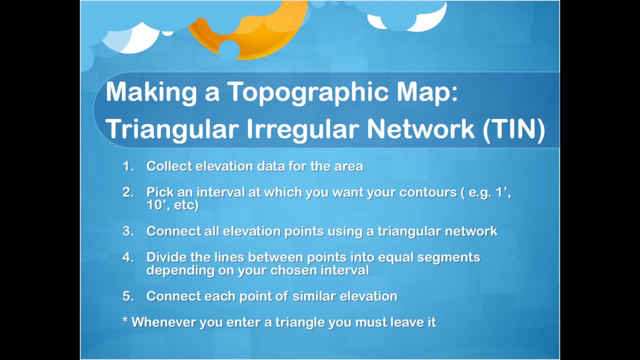 In the final step, the points with equal elevation are connected to form a smooth contour line. When drawing the contour lines in the fifth step, it's important to remember that the points with equal elevation are connected to form a smooth contour line. Remember that you must leave every triangle that you enter. 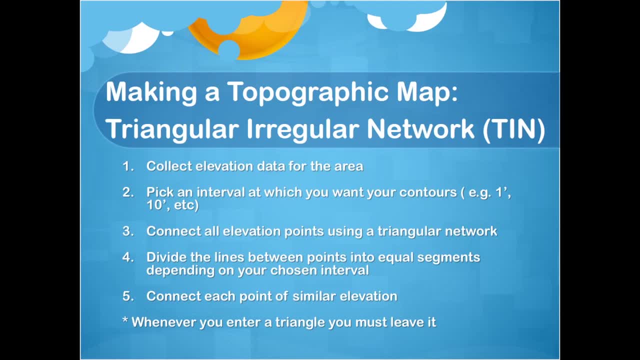 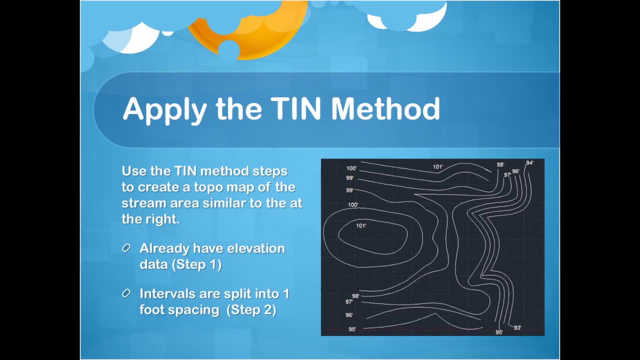 In other words, you can't have a contour line that just ends abruptly. Let's go through the TIN method to create a topo map like the one shown on the right side. We already have elevation data and, since it's a relatively small region, 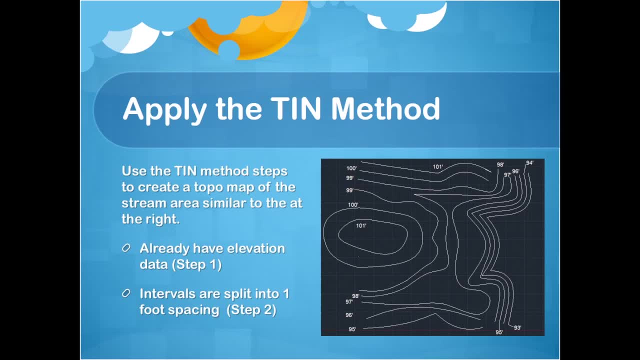 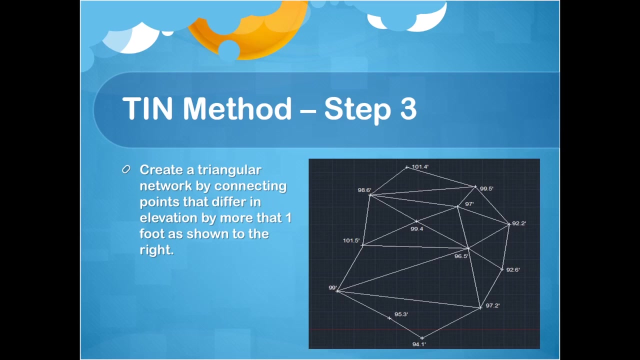 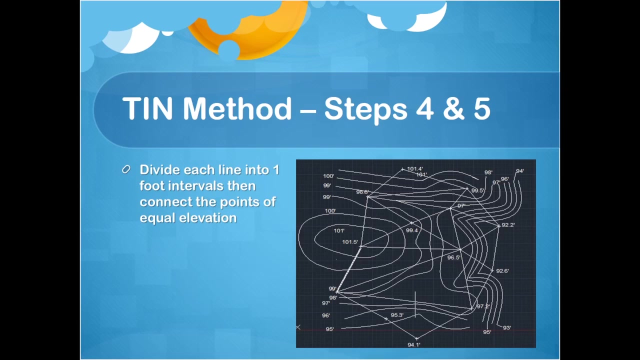 we will use 1 foot intervals. so the first two steps are complete. What should we do next? We create a triangular network by connecting points with different elevations. Now we're ready for the fourth step. In the fourth step, we divide each of the lines between the points using the 1 foot interval. 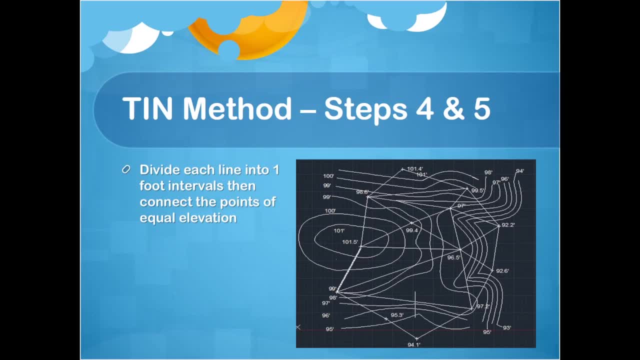 Each time we mark an interval, we make a small hash mark that's perpendicular to the line. Then, in step 5, we connect all the hash marks that represent the same elevation. Once we've finished connecting the hash marks, we have our contour lines for our tip of the line. 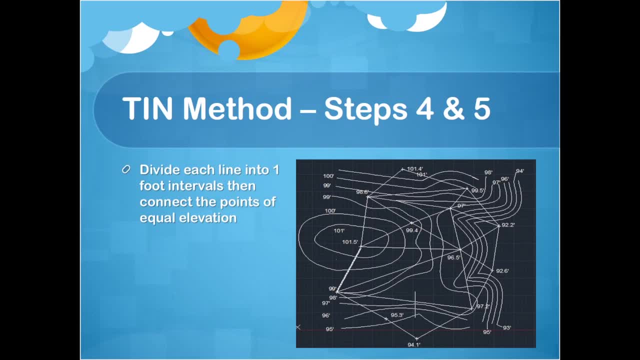 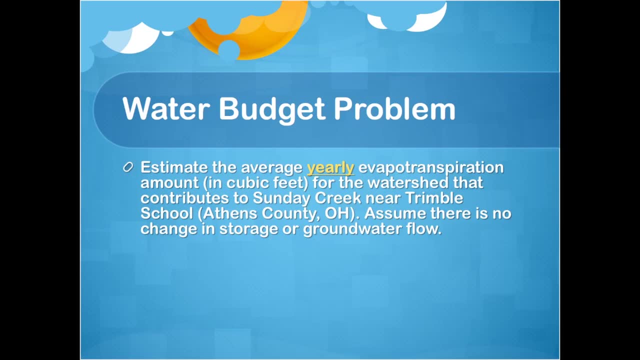 Now that we have an understanding of watersheds and topo maps, let's try a water budget problem. We want to estimate the average yearly evapotranspiration amount in cubic feet for the Sunday Creek watershed near Trimble High School in Athens County, Ohio. 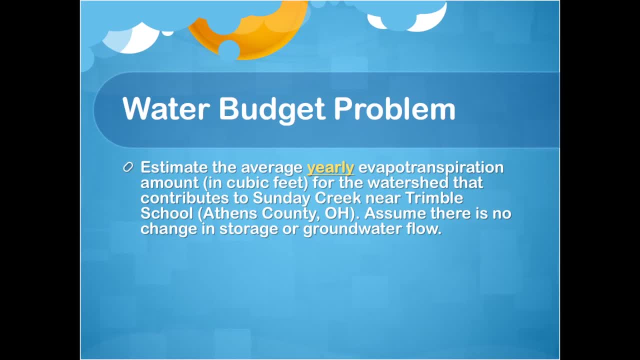 We will assume no changes in storage or groundwater flow. Take a minute and try to write out the water budget equation that we will use to solve this problem. Remember that the water budget equation is precipitation plus change in stream, discharge minus evapotranspiration plus change in groundwater flow equals change in storage. 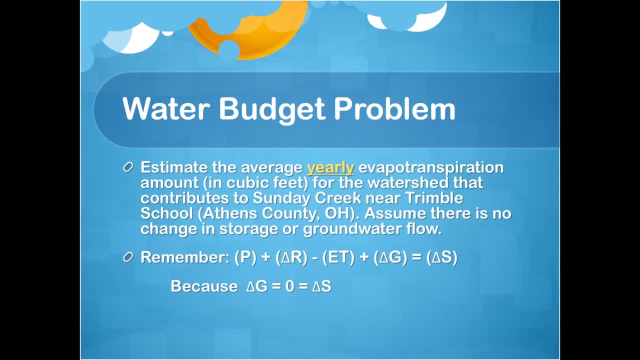 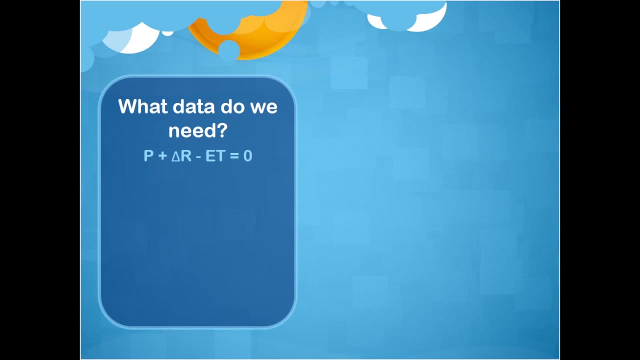 But we said no changes in storage or groundwater flow, So delta G and delta S will be set equal to zero, which means we can use the simplified version of the equation: P plus delta R minus ET equals zero. So what data do we need in order to solve this problem? 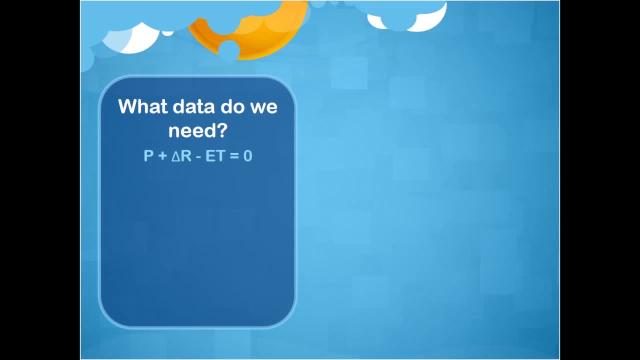 Remember our equation We're trying to solve for ET, so we need values for precipitation and stream discharge. We'll also need to know the watershed area so we can convert the evapotranspiration amount from cubic feet to inches. The values that we will use to solve this problem are: 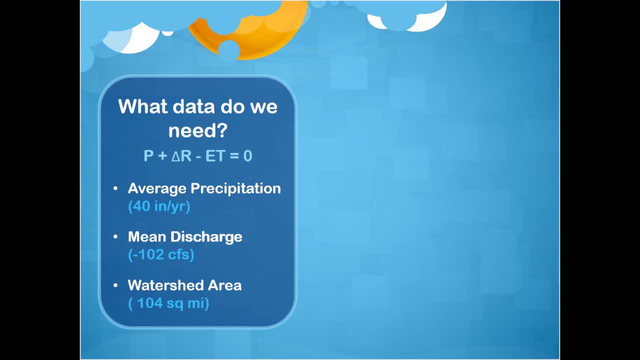 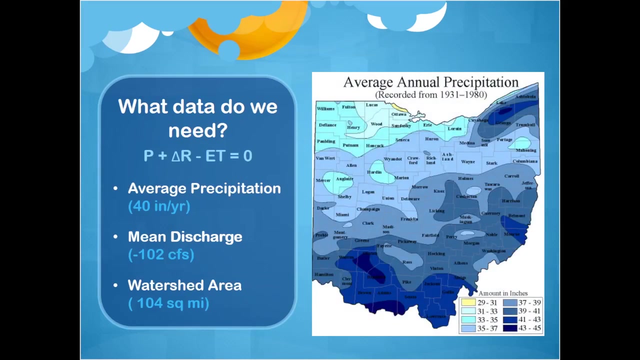 40 inches per year for average precipitation, negative 102 cubic feet per second for stream discharge and 104 square miles for watershed area. Let's go through the steps for determining the values for each term. To find the average precipitation, we can reference historic precipitation information. 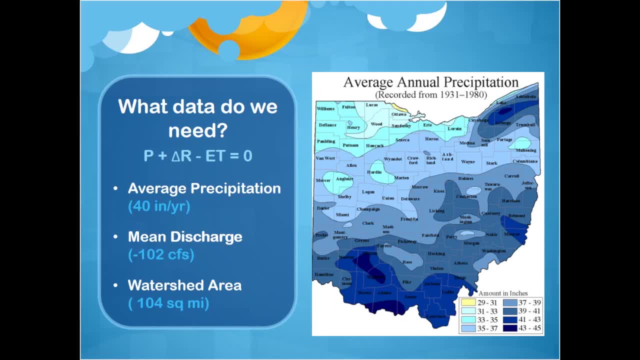 We can use this average annual precipitation map, knowing that Sunday Creek is located in Athens County, to find the average precipitation is between 39 and 41 inches per year. We'll use an average value of 40 inches per year for our calculations. 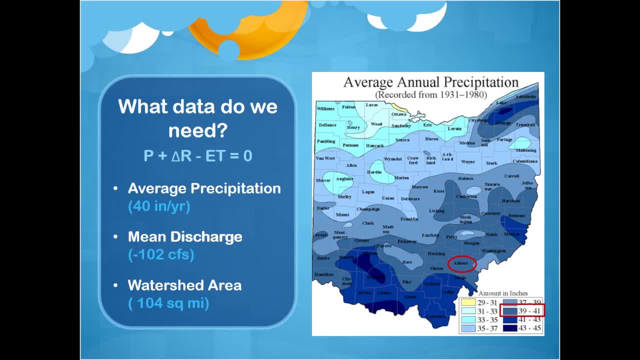 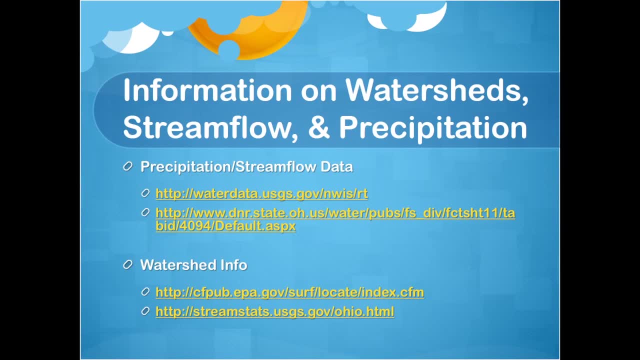 To find the mean discharge and watershed area we'll have to use some external sources. We can find information about precipitation and stream flow from the USGS Water Data website or from the Ohio Department of Natural Resources website. We can get watershed information from the EPA website. 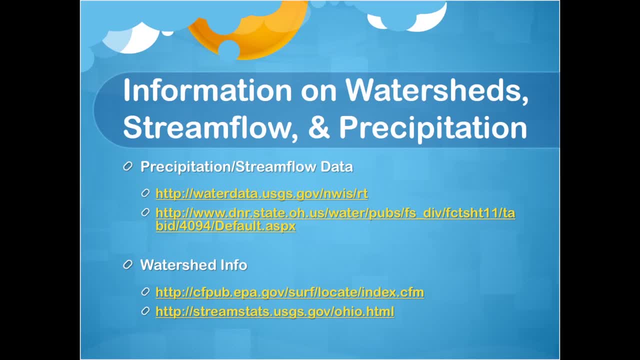 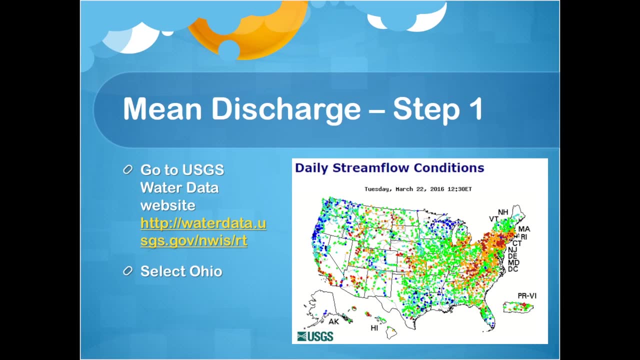 or from the USGS Interactive Stream Stats map. Let's start by finding the mean discharge and then determine the watershed area. Start by going to the USGS Water Data website. by following the link shown and select Ohio from the map, You'll be redirected to another page for Ohio stream flow. 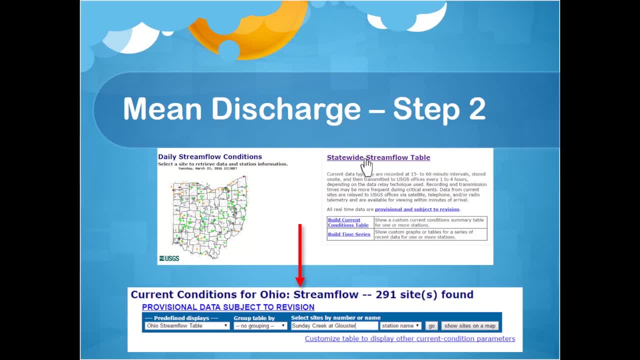 On this page, click the link for the statewide stream flow table. You'll be taken to another page where you can select the site Type in Sunday Creek at Gloucester. On the next page, click on the station number for Sunday Creek at Gloucester. 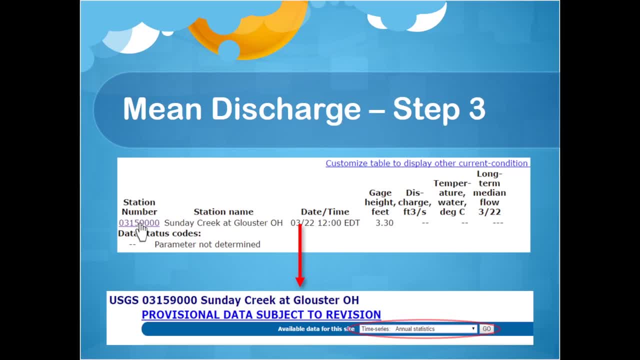 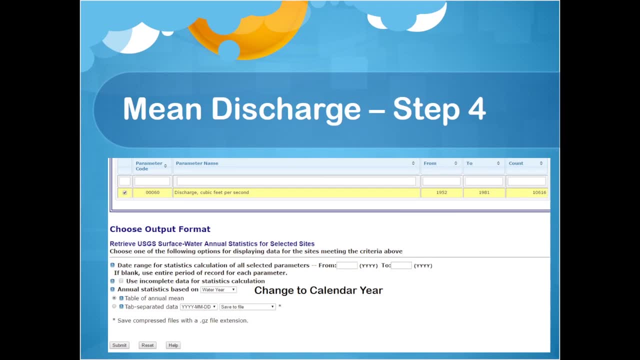 You'll be redirected to another page where you should select annual statistics from the drop-down menu for available data. You will then be prompted to select the output format for your table. Make sure to check the box for discharge and change from water year to calendar year. 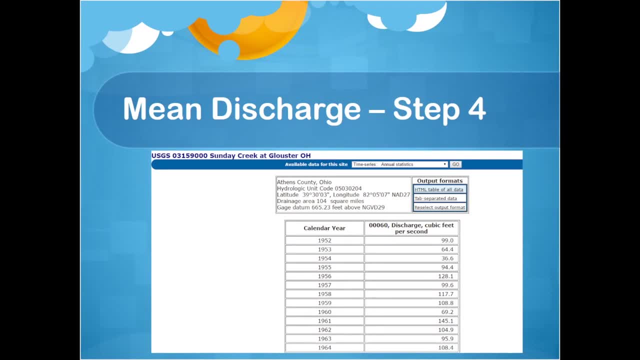 Then submit. The website will give you a table with the stream discharge data for each year. We'll take the average of the discharge data in the table to get the mean discharge, which comes to approximately 102 cubic feet per second. We're going to make this amount negative in the water budget equation. 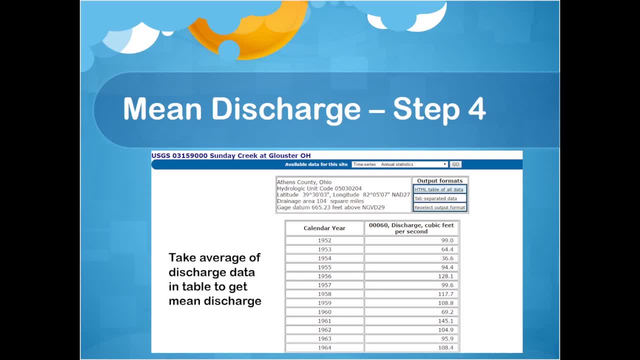 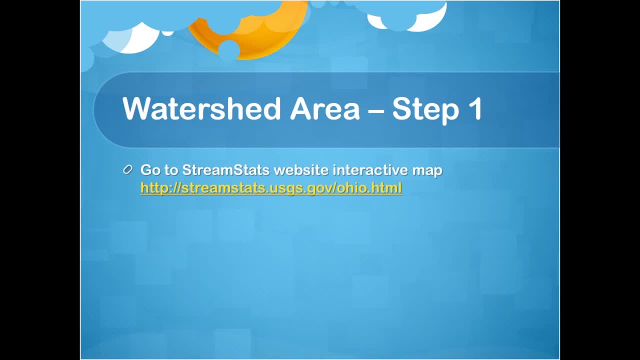 because it represents discharge water. leaving the system Now, we'll determine the watershed area by using the USGS Stream Stats interactive map. Once you've entered the interactive map user interface, zoom to Gloucester Ohio. You'll get an image on the map like this: 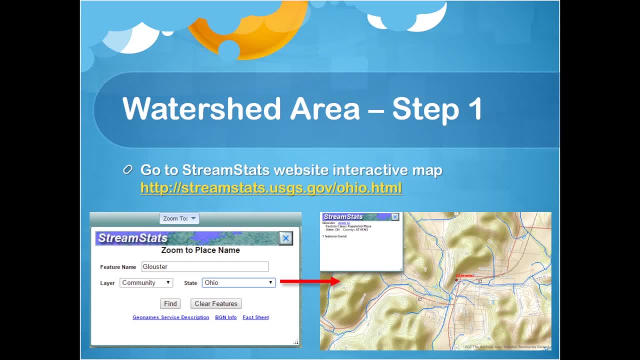 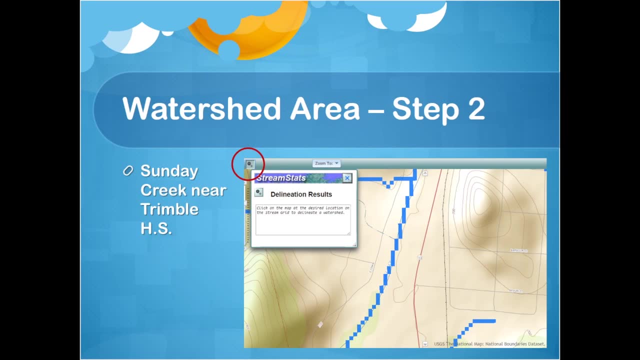 that shows Gloucester and surrounding creeks and roads. Next, select the watershed delineation from a point tool, Zoom in on the map to Sunday Creek at the point where it runs past Trimble High School and click on the stream After the tool finishes calculating. 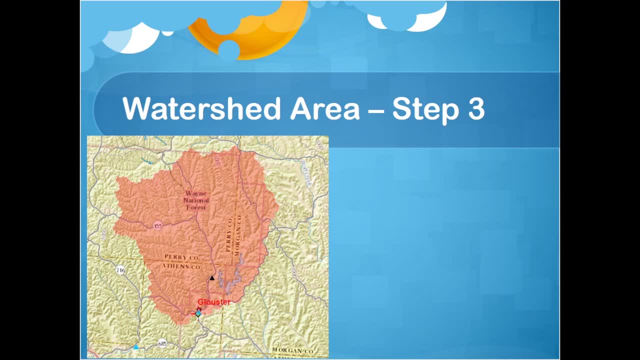 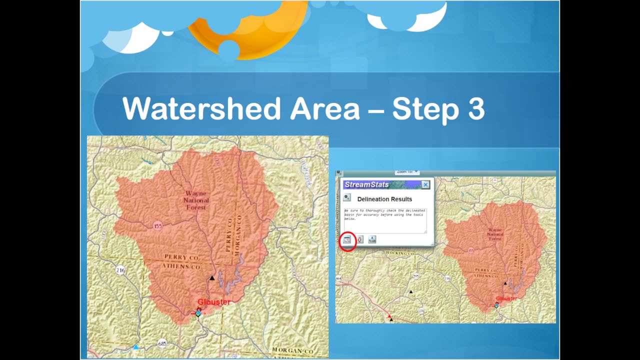 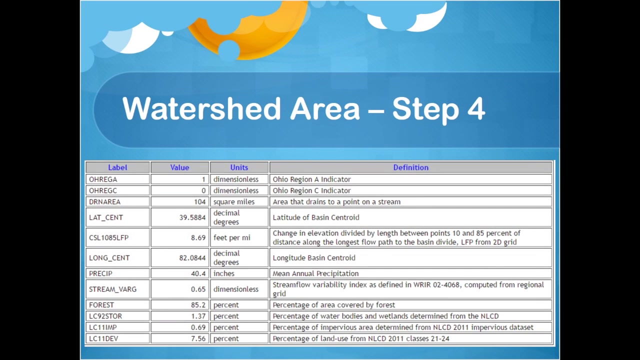 the watershed will be highlighted on the map in red. With the delineation tool still open, click the Compute Basin Characteristics button. Leave the default selections in the pop-up window and click Compute Basin Characteristics From the table of basin characteristics that's generated. 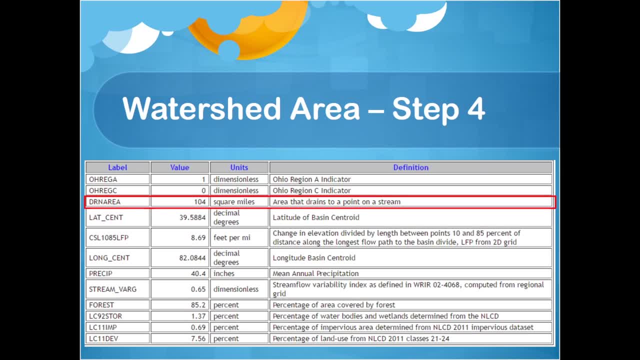 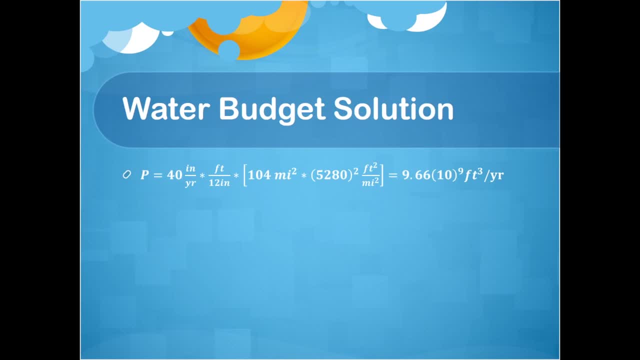 we can find the drainage area to be 104 square miles. Now we have everything we need. in order to complete the water budget calculation, We'll start by converting the precipitation value from inches per year into cubic feet. We'll do this by multiplying the watershed area. 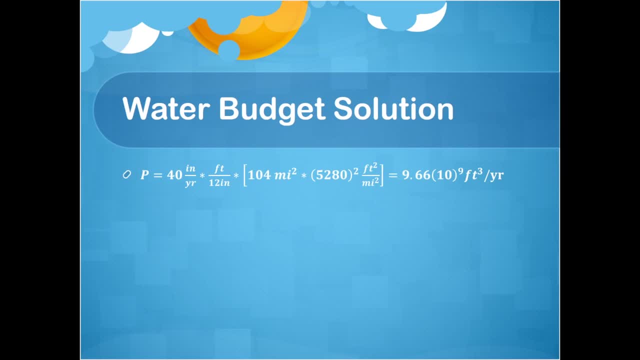 by the average precipitation. Remember to include conversions from inches to feet and from square miles to square feet. Next we'll convert the stream discharge from cubic feet per second to cubic feet per year. Now we can calculate the evapotranspiration as precipitation minus stream discharge.